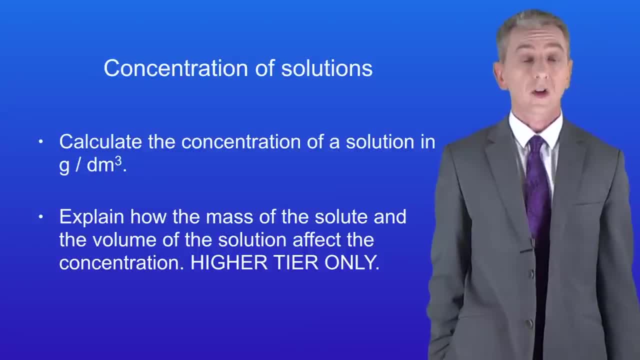 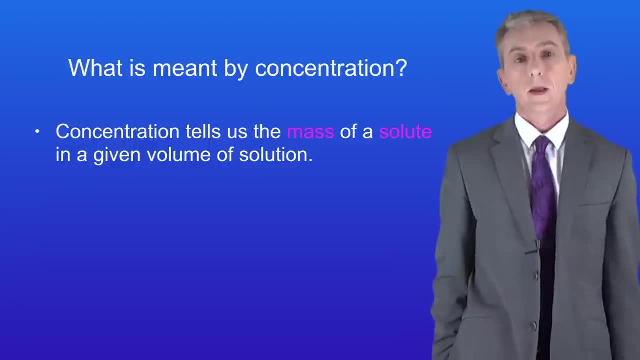 the concentration. So let's start by looking at what's meant by concentration. The concentration tells us the mass of a solute in a given volume of solution. Now I should point out that if you're a higher tier student, you learn another definition of concentration, as well as this one, in a later. 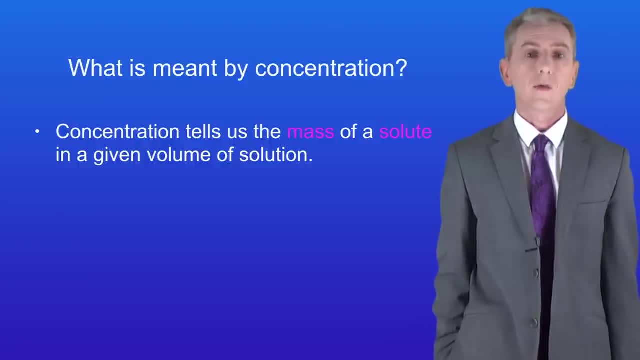 video, But if you're doing foundation, then you only need to learn this definition. So what's meant by a solute? Well, a solute is a chemical which is dissolved in a solvent, and in chemistry, water is often used as a solvent. The unit of concentration for this definition is grams per 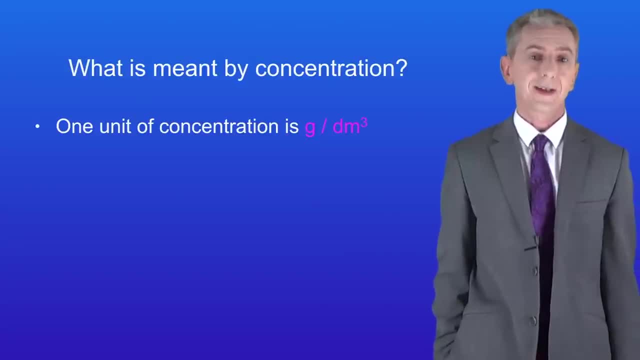 decimetre cubed. A decimetre cubed is what used to be called a litre, but scientists don't use that word anymore. Now we calculate the concentration using this equation. This equation is not in the spec, but I do think it's worth learning. The concentration in grams per decimetre cubed is: 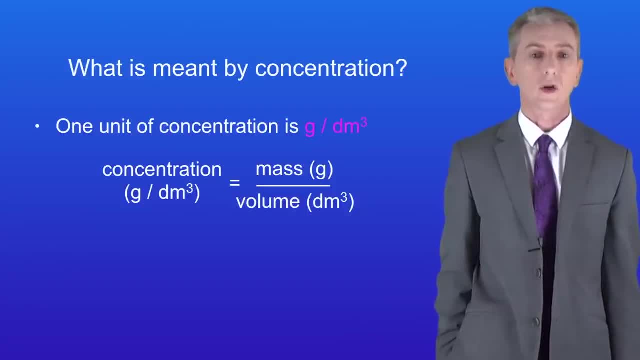 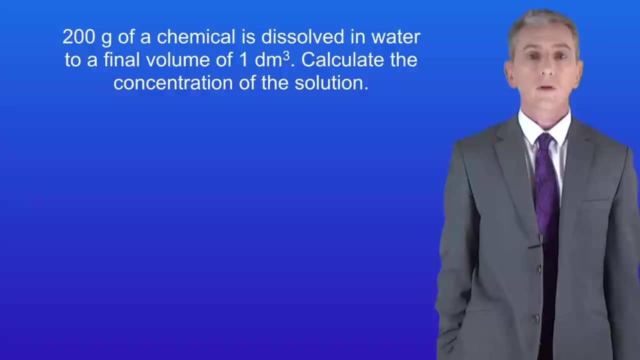 the mass in grams divided by the volume in decimetres cubed. And here's a triangle to help you learn this. So let's look at a typical question. 200 grams of a chemical is dissolved in water to a final volume of one decimetre cubed. Calculate the concentration of the solution. 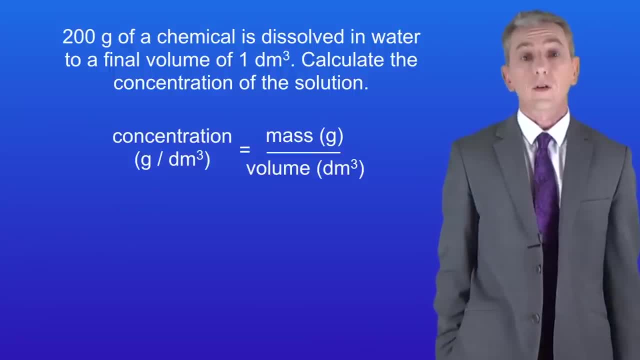 Here's the equation To find the concentration: we divide the mass in grams by the volume in decimetres cubed. This gives us a final concentration of 200 grams per decimetre cubed. Now, that was quite an easy one, so let's look at something a bit more challenging. 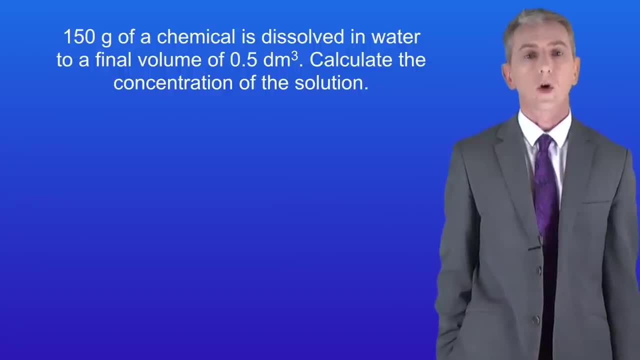 150 grams of a chemical is dissolved in water to a final volume of 0.5 decimetres cubed, Calculate the concentration of the solution. Pause the video and try this yourself. Okay, dividing 150 grams by 0.5 decimetres cubed. 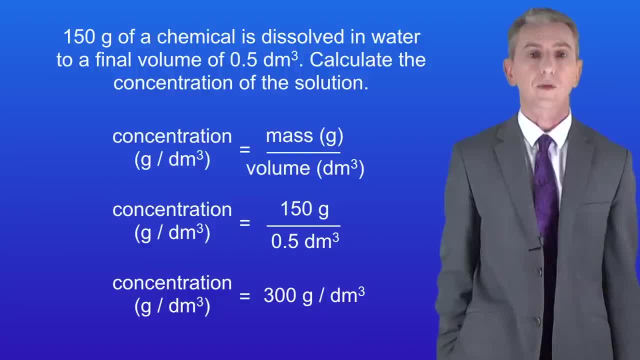 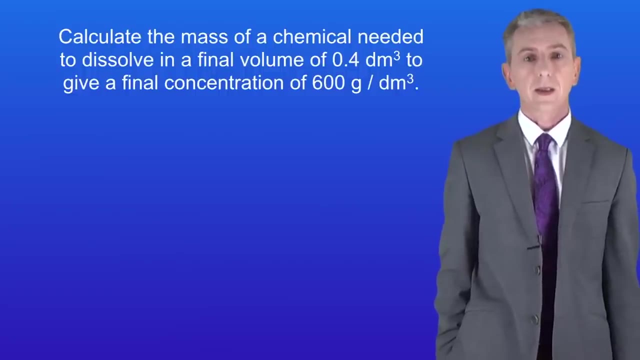 gives us a final concentration of 300 grams per decimetre cubed. Okay, now in the exam you could be asked to rearrange this equation and calculate the mass of a solute or the volume of a solution. So here's another question for you: to try Calculate the mass of a chemical needed to 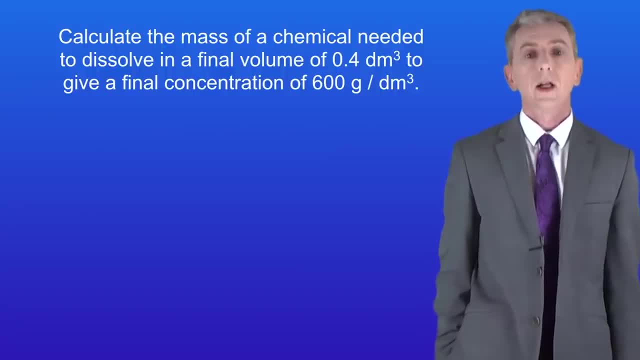 dissolve in a final volume of 0.4 decimetres cubed to give a concentration of 0.5 decimetres cubed of 600 grams per decimetre cubed. Now to answer this question, it's worth using the triangle Pause.